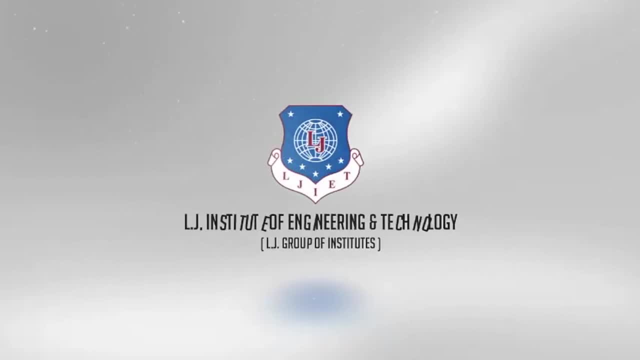 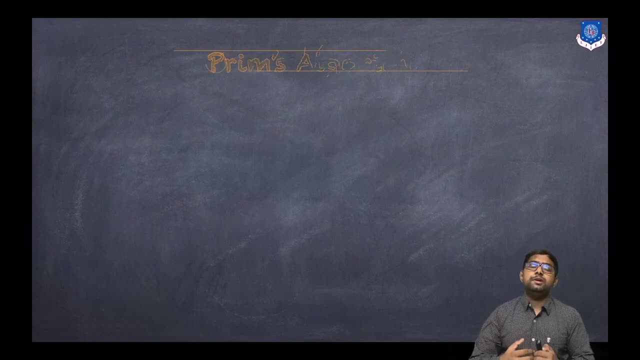 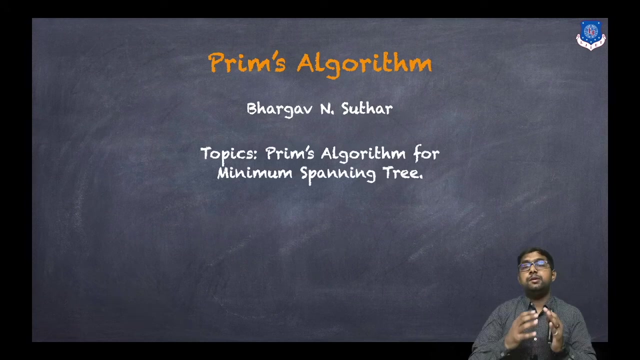 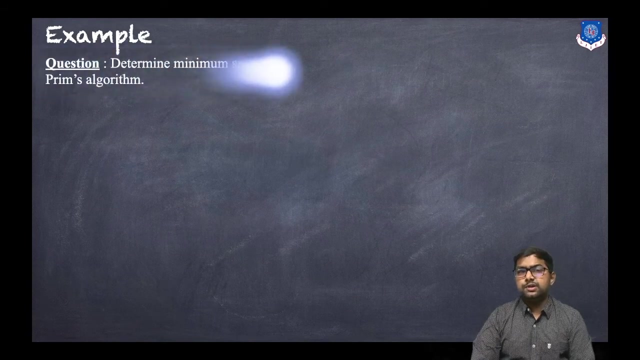 Hey everyone, this is Pargav Suthar, and today we will learn very important algorithm, so that is Prim's algorithm. So in this session we will discuss how to find a minimum spawning tree using Prim's algorithm. Okay, now see, let us directly jump to the example. So determine. 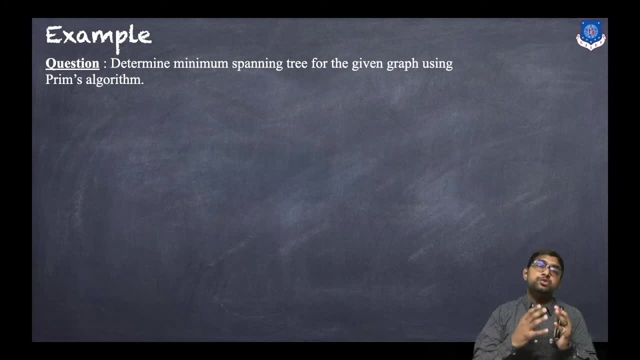 the minimum spawning tree for the given graph using Prim's algorithm. Okay, so, first of all, what is a spawning tree, and then what is a minimum spawning tree. So, what is a spawning tree? and for that, what is a tree? So it is a acyclic graph, So that is a tree. Now, what is a spawning tree? 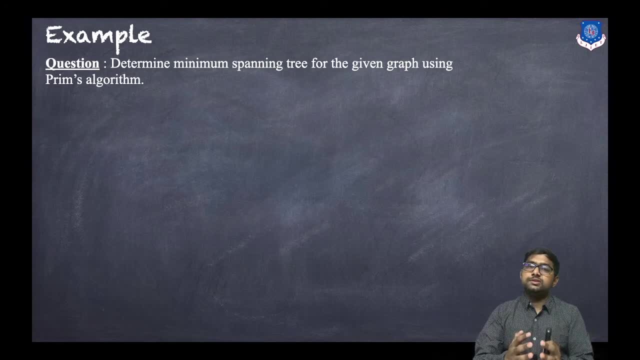 So it is a tree in which it covers all the vertices, Okay, in such a manner that all are connected. Fine. and what is a minimum spawning tree? So it is a spawning tree having the minimum weight, Fine. So we will use this Prim's algorithm to find a minimum spawning tree, or that is, MST. 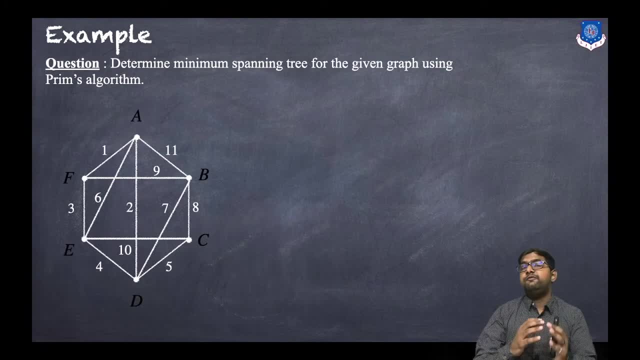 Okay, so this is the example, Okay, and we want to find the minimum spawning tree of this particular example, So let us do that. So see, I am not talking about the. what are the steps to be followed? So, first of all, what we will do. Okay, so here, first of all, how many vertices are there? 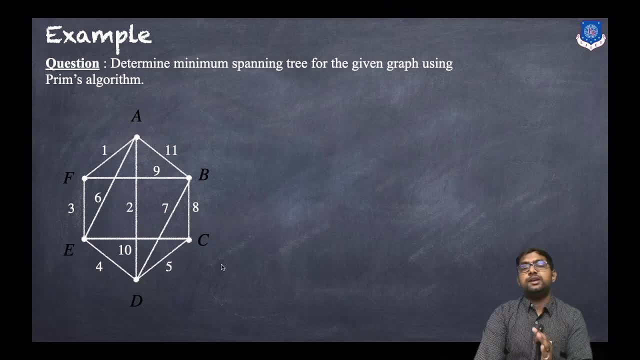 So, total, you can see that there are six vertices. Fine, So we can start from any one vertex. Okay, to proceed further, this method or the algorithm, we can start from any vertex. Fine, So for simplicity, I will just start from this: A. 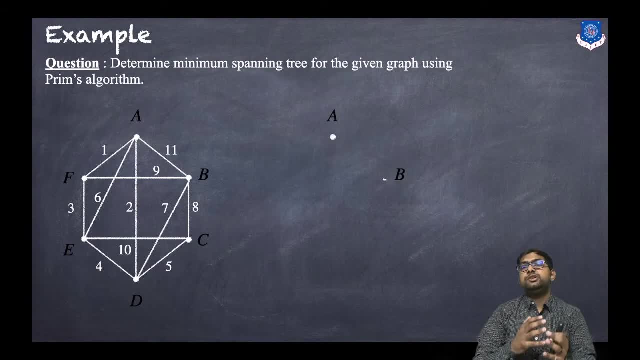 Okay, see, as it is a spawning tree, So it should contain all the vertices. Fine, So what we will do? just take all these vertices, that is, A, B, C, D, E, F. Okay, so we have taken all the vertices. So what is the first step Now? we will start with A, Now from A, or with A. 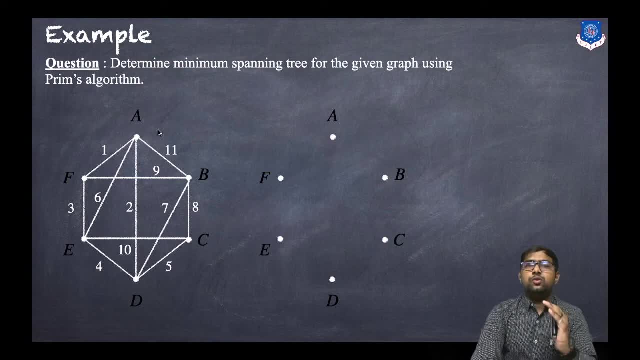 We will select a minimum weighted edge or minimum weighted vertex which is adjacent to A. So, first of all, what are the adjacent vertices? So that is F, E, D and B. So what is the minimum weight? So, as you can see that we have this: 1, 6, 2 and 11.. So, among all this four, what is the minimum weight? 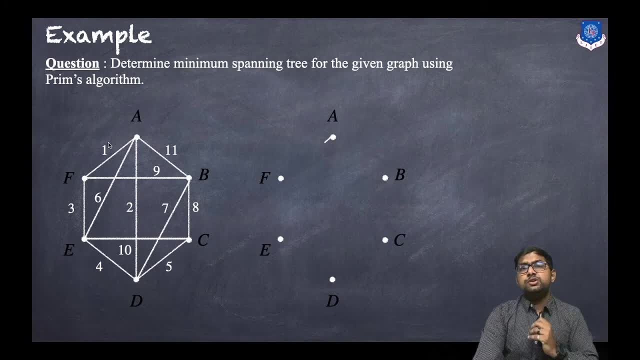 So, as you can see that this 1 it is the minimum weight. So what we will do, we will just draw this edge and we will write This weight 1.. Fine, Now the second step. Okay, so we will choose the third vertex in. 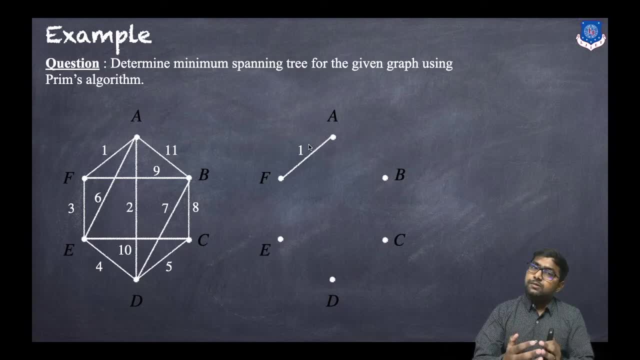 such a manner that it is the minimum. Okay, it is the minimum weight and as well as it should not contain a cycle, as we are finding the minimum spawning tree, So obviously it should not contain, or it should not become a cycle. Fine, So the second step is that 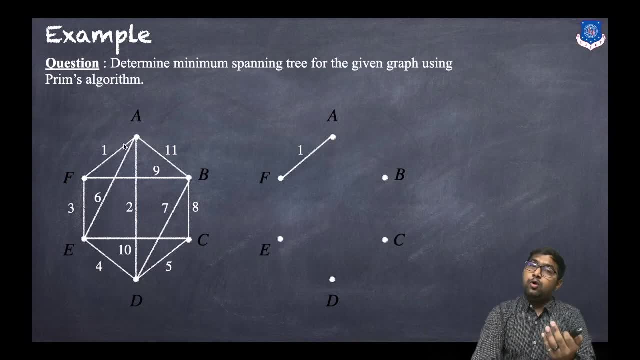 we will check for all these, both the vertices. Fine, So we will check for both the vertices, that is, F and A. Now we will take third vertex by using this two vertices. So that is now what is the minimum weighted vertex. Okay, So our minimum weighted adjacent vertex. So what are the vertices? 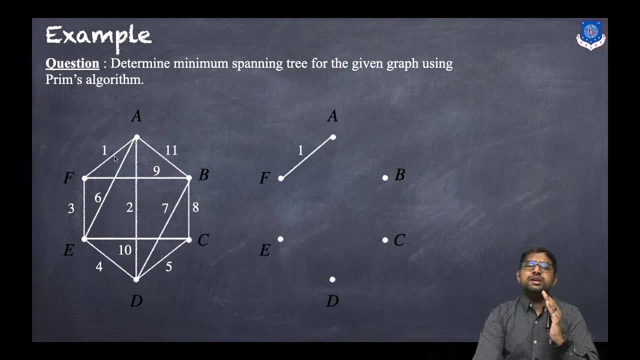 adjacent to F. So that is this E and B. Now we've already taken this A, So E and B. So weight is 3 and 9.. And for A, The 6, 2 and 11.. So 6, 2, 11 and 3 and 9.. So we will consider. 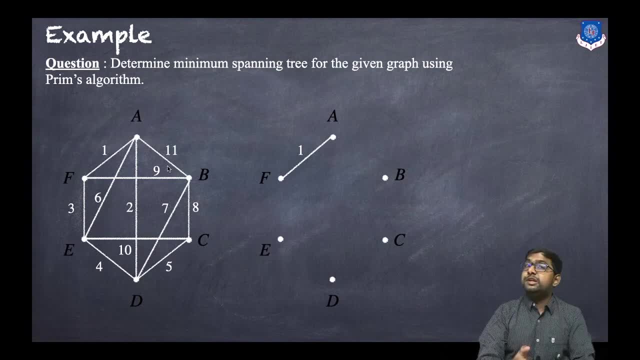 both the vertices. Fine. so among all these, what is the minimum weight? so that is 2. so, as you can see that it is 2, so we'll select this vertex D and draw this a edge. this 2: fine. so this is the second step. so that is 2 and D. okay, now the third step. so what we'll? 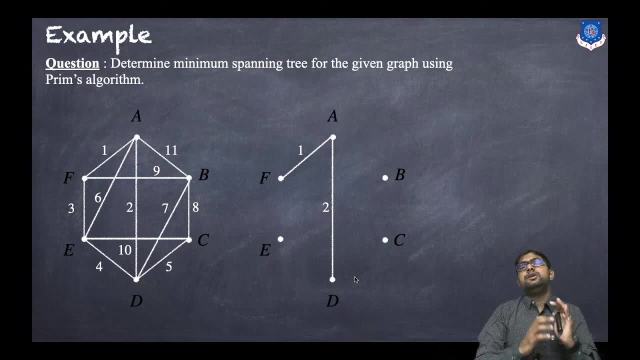 do now we'll look for this F, a and D. so we'll take that vertex which is minimum weighted, fine, from all these three vertices, the adjacent vertices, fine. so now just consider this F. so what are the vertices? that is a that has minimum weight, or this edge has minimum weight. so that is this 3. okay, so this is 3 now. 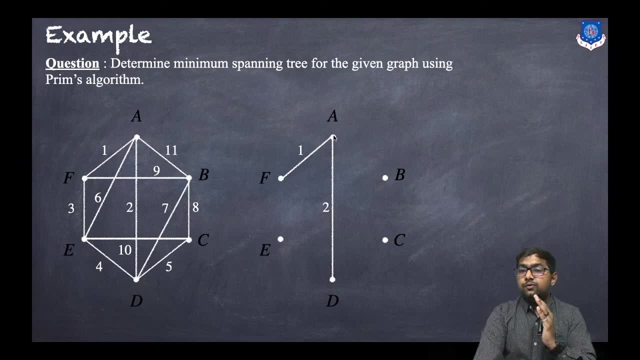 this is 9, so just consider 3 and 9. now, what are the adjacent edges? that is a, so one. I've already taken 6 and 11. so 6, 11, 3, 9 and for D, for D, we have 4, 5, 7, okay, so what is this minimum? so, as you can see that this 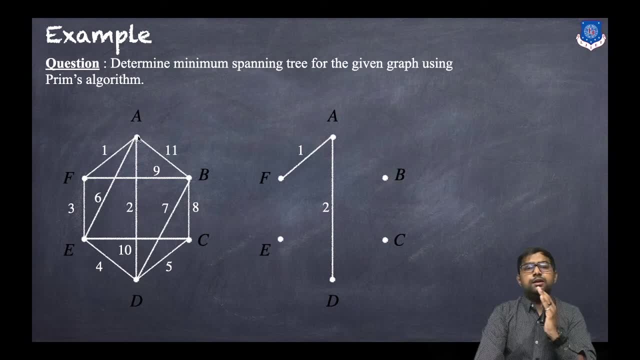 3, 9. here for F, 3, 9. for a, we have 6, we have 11, and for D, we have 4, 5, okay. so what is this minimum? so that is this 3, okay. so what we'll take, we will take. 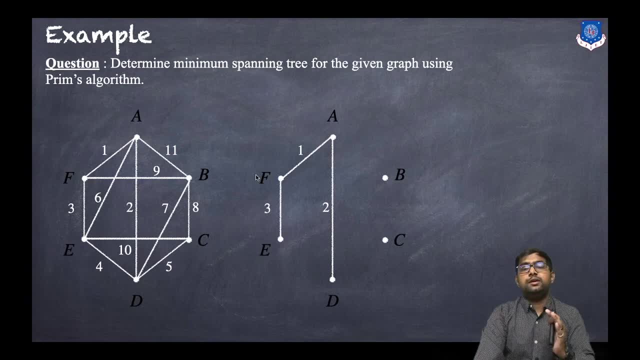 this 3. fine, so we'll take this 3, okay, now. next step. now what we'll do? we have total 4 vertices, so we'll check for all the adjacent edges, okay, and which has the minimum weight. so for a, we have this 11 and 6. okay, for F, we have this 9. only 9, 9 is left. so then next for. 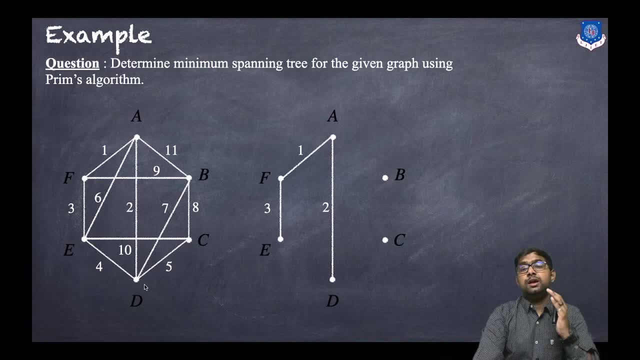 E, we have this 10, we have 6 and 4. fine, and for D, we have 5, we have 7. okay, so just just by looking at this you can see that this 4, it is the minimum. but see if we take this 4 or if we take this edge E D, so if we take this E D, so it 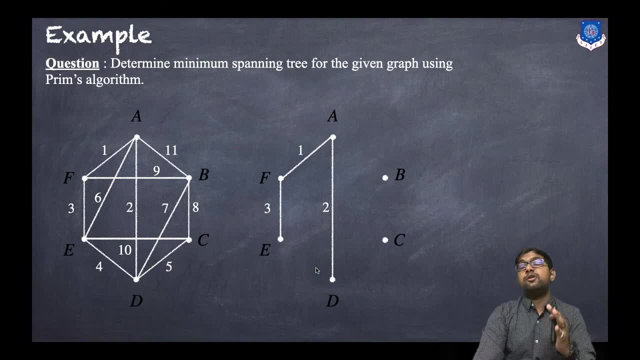 will become a cycle. but what we are looking for, we are looking for a tree, so it should does it should not contain a cycle, fine, so this for this edge won't be there. so what is this next minimum weight? so the next minimum weight is, as you can see, that this is 5. okay, so we'll take this D and C, so that is 5, fine. the 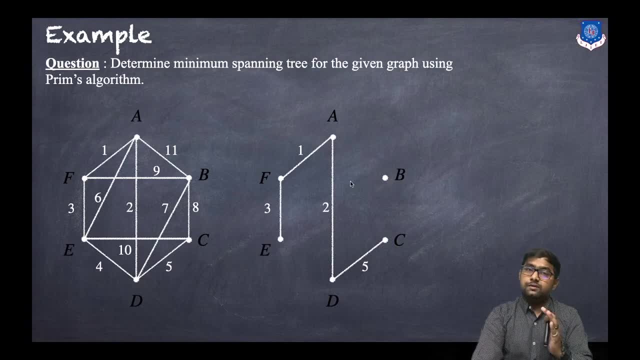 next step. now again, we have total 5. we have total 5 vertices. now we'll check for each and every adjacent edges such that it has the minimum weight. so for a, we have this 11 and 6. fine, for F, we have this 9. yeah, only 9. then we have. for E, we have 6, then we 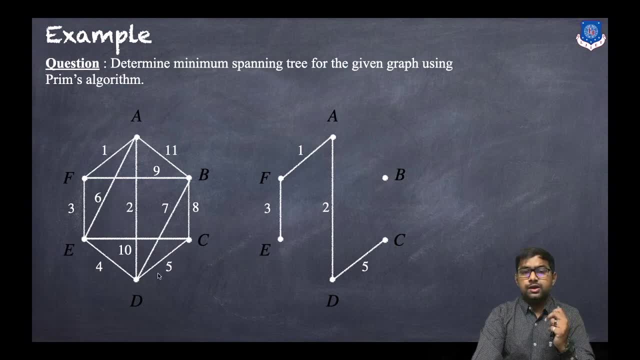 have this 10 and 4 cannot be there, okay. and for D, we have this 5 already taken and 7, okay. so what will be it? so? and then for C, we have this 8, or that means this busy BCH, okay. so what is this minimum weight? so, as you can see that, this minimum,